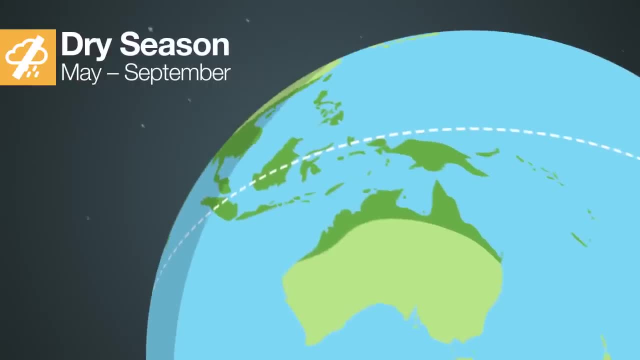 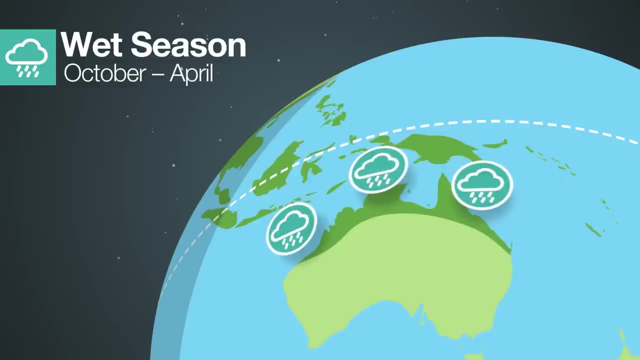 including northern Australia. In northern Australia, we have two distinct seasons: a dry season, which roughly coincides with the southern winter, and a wet season which peaks during the summer months, When an active monsoon arrives that the sky is filled with dark clouds, we see widespread rain. 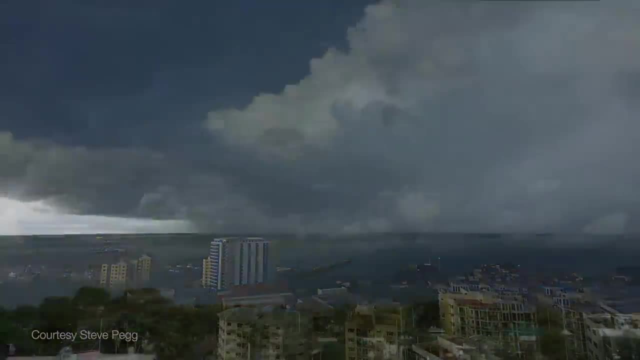 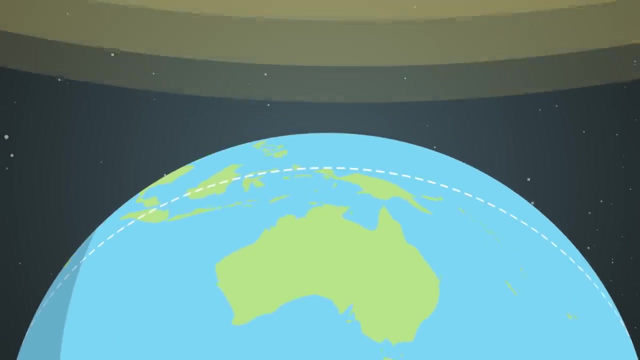 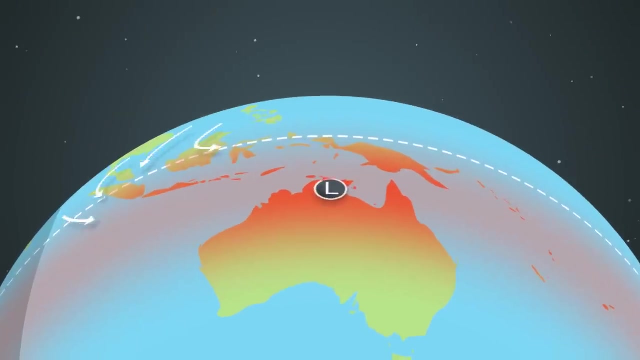 showers and thunderstorms, and these can last for a few days or even a week or more. The Australian monsoon develops in response to summertime heating over the northern Australian region. when the continent warms at a faster rate than the surrounding oceans, This sets up a giant sea. 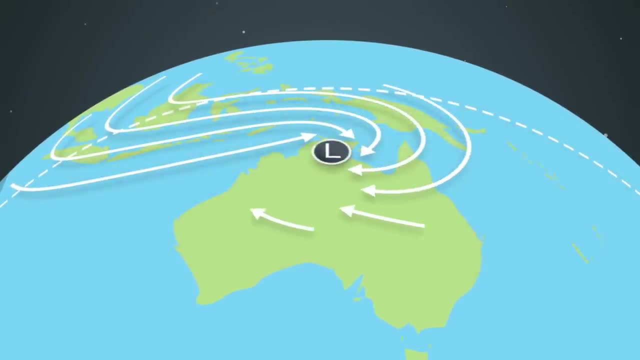 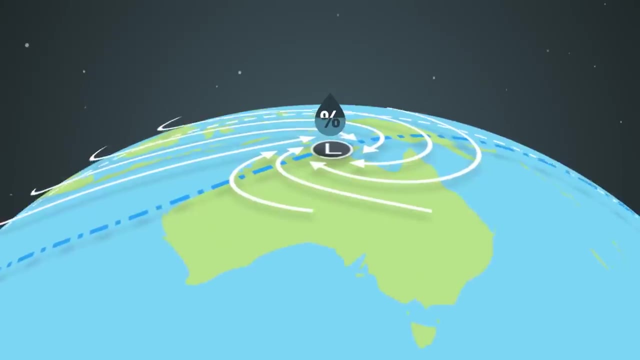 breeze circulation drawing in monsoons. The monsoon is a common monsoon in Australia and moisture from these oceans over the lower pressure on the land As the humidity progressively builds a monsoon trough, which is the focus for the rainfall, and cloudiness becomes established. 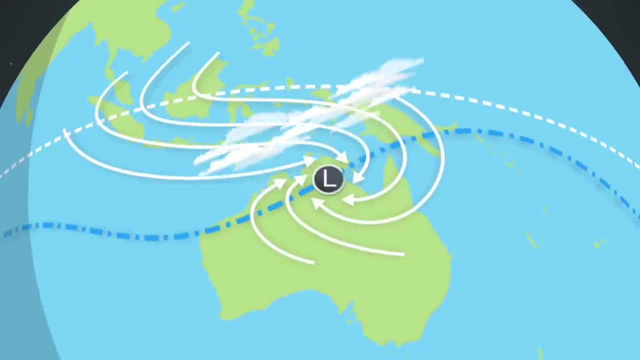 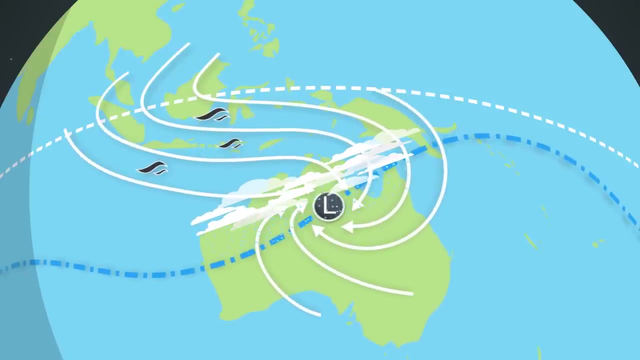 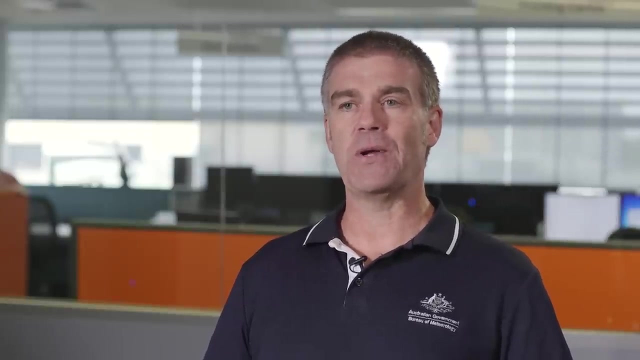 over the Australian region. True monsoonal flow with deep low-level westerly winds exists north of the trough, so when the trough moves south over a location, this area becomes affected by monsoonal conditions. An active monsoon period can be followed by an inactive or break monsoon period. 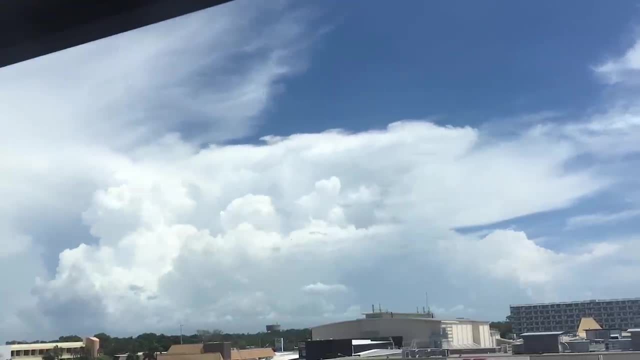 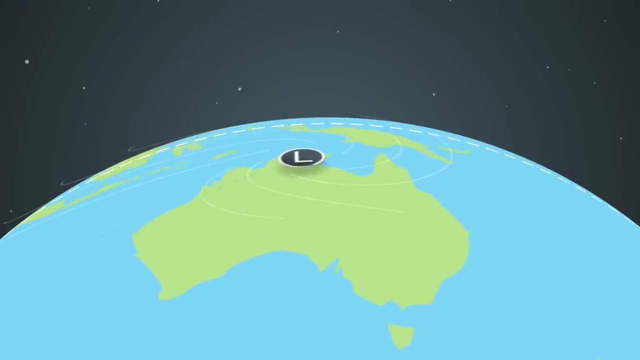 when we return to the south of a location. This is when we return to the south of a location. Northern Australia typically sees about three monsoon bursts each wet season sometimes occurring as late as mid-April. The end of the final monsoon burst of the year is called. the monsoon retreat. Before the onset of the much anticipated monsoon, northerners endure the so called build-up, a time when we can go a bit troppo due to the extreme heat and humidity. The cooling the monsoon rains provide welcome change from the build-up and herald the annual transformation from. 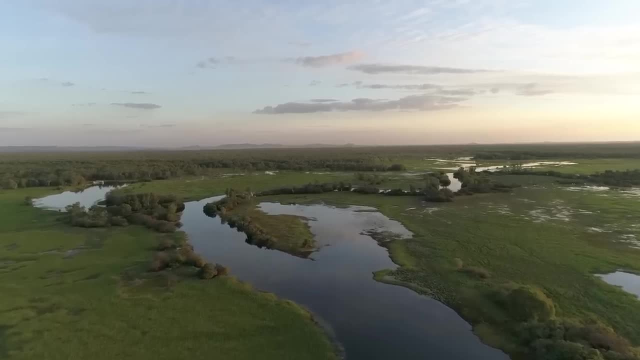 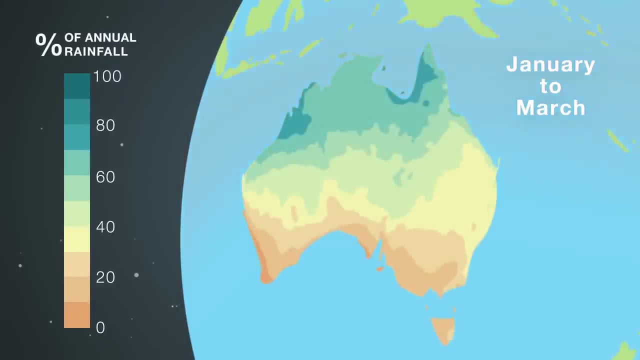 a dry brown landscape to a lush watery oasis. It's these monsoonal rains that deliver the vast majority of the annual rainfall across most of tropical northern Australia. Farmers, communities and the ecosystems which have evolved across Australia's north depend on these monsoonal. 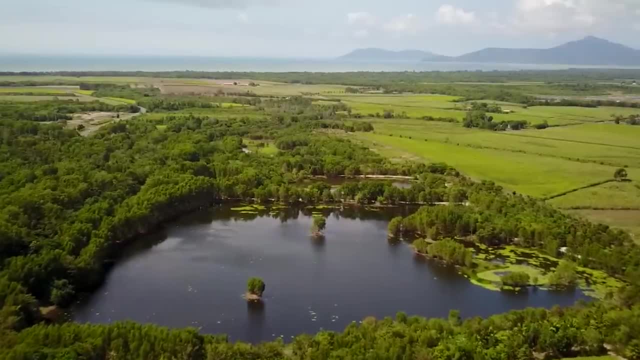 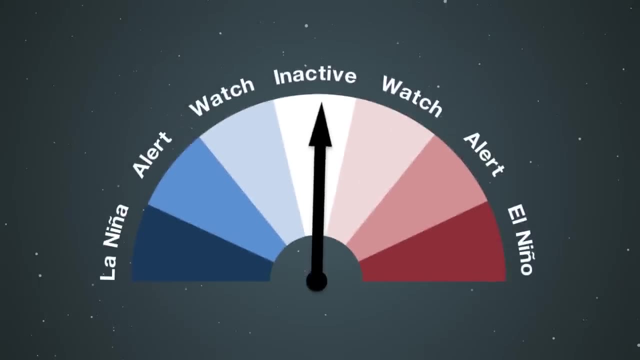 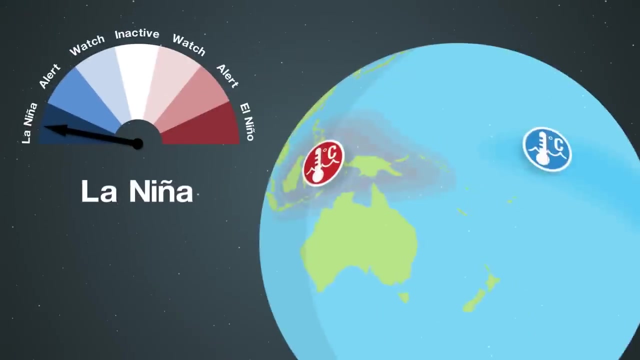 rains to replenish water storages and recharge natural aquifers. These rains can, of course, create substantial flooding and restrict movement across large areas. Climate factors, such as whether it is El Niño or La Niña, can have a significant impact on monsoonal variability. La Niña typically means 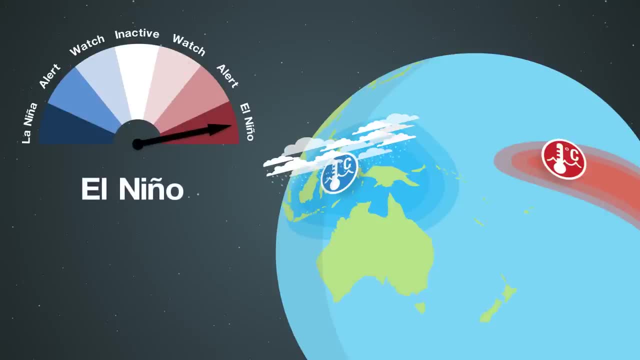 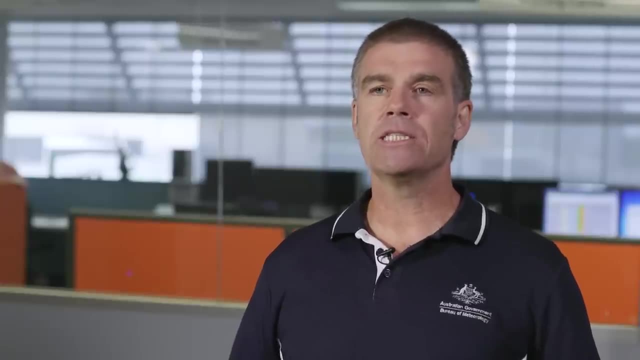 earlier than normal monsoon onset, while El Niño is often associated with rainfall during the monsoon season being less than average. Another important climate driver is the Madden-Julian Oscillation, or MJO. It can have a significant impact on the timing of the active and inactive.